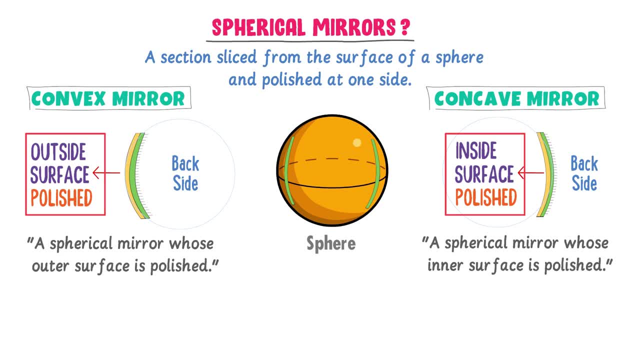 While in concave mirrors the inside surface is polished. Also, let me teach you that why concave and convex mirrors are called spherical mirrors. It is because both concave and convex mirrors came from a sphere, or they both are made out of a sphere. 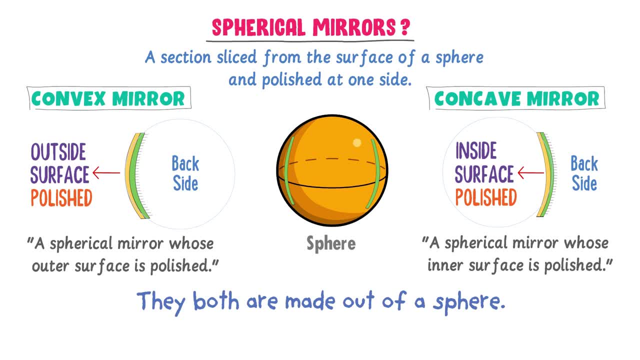 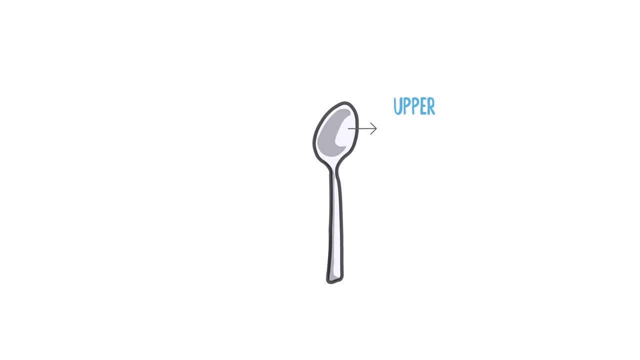 So they are therefore called spherical mirrors. Now the easy trick to remember the concave and convex mirrors is the spoon. The upper part of the spoon is just like a concave mirror and the lower part of the spoon is just like a convex mirror. 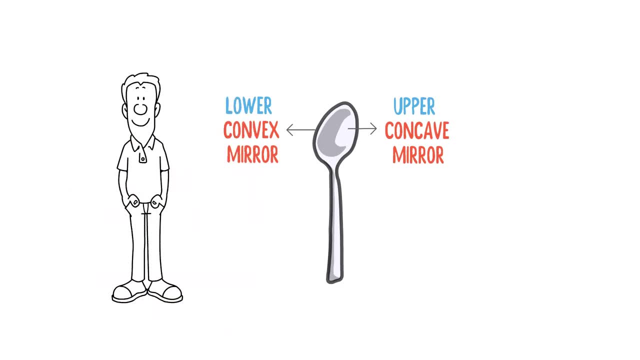 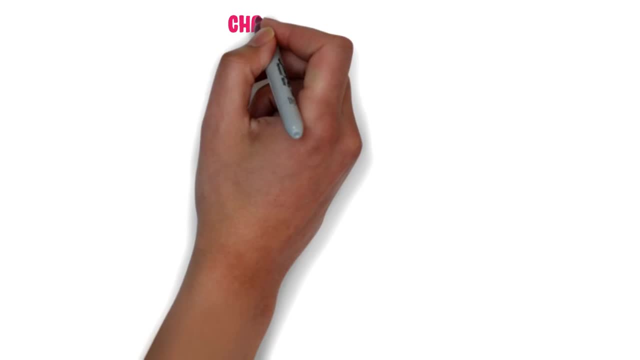 You can do this simple experiment at your home by looking into the upper and lower part of the spoon in order to see your face image in it. Now let me teach you the characteristics of a concave and convex mirrors. Let's consider concave and convex mirror. 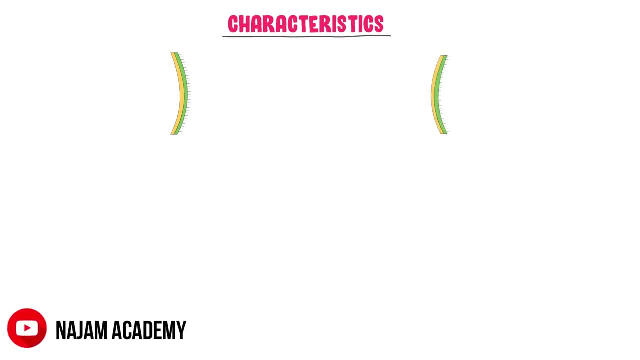 We know that concave mirror is a part of a sphere and convex mirror is also a part of a sphere. Thus I draw these imaginary spheres around them. Firstly, what is center of curvature? The center of a sphere is called center of curvature. 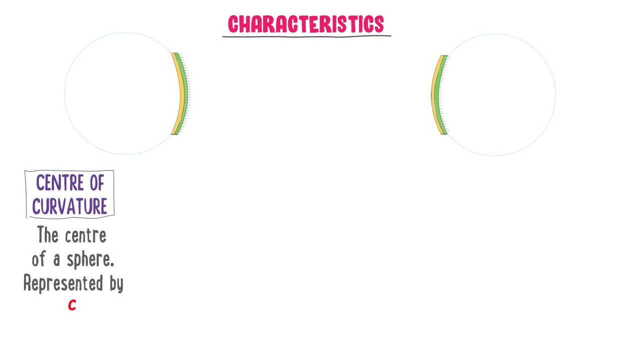 It is represented by C. In case of concave mirror, this is the center of a sphere, So it is the center of curvature of a concave mirror, While in case of a convex mirror, this is the center of a sphere. 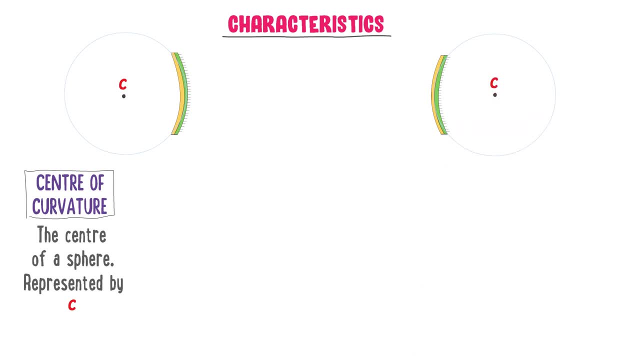 So it is also the center of curvature of a convex mirror. Secondly, what is pole or vertex? The midpoint of a mirror is called pole or vertex. It is represented by P. For example, this is the midpoint of the concave mirror. 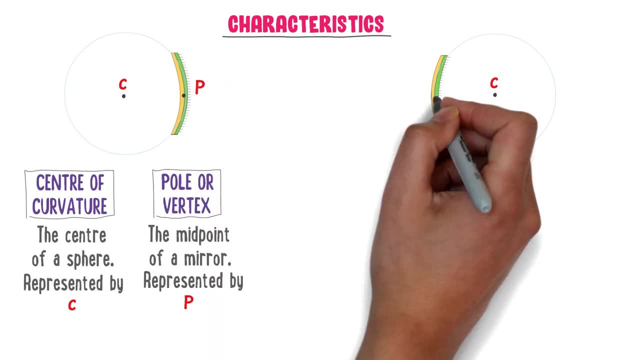 So it is the pole or vertex of a concave mirror, While this is the midpoint of a convex mirror, So it is the pole or vertex of a convex mirror. Thirdly, what is radius of a curvature? The radius of a sphere is called radius of a curvature. 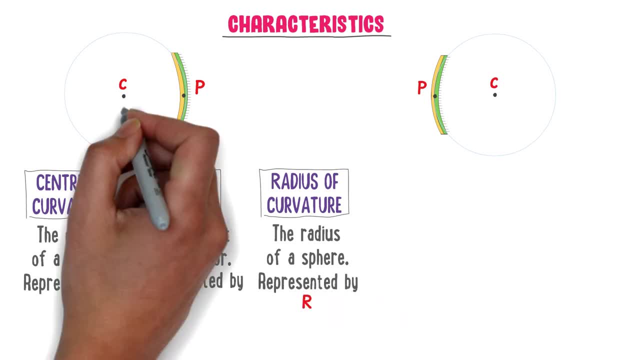 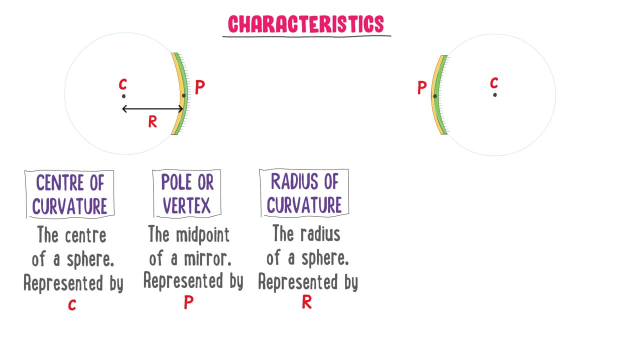 It is represented by R. For example, the distance between the center of curvature C and pole P is called radius of the curvature R of a concave mirror, While the distance between the center of a curvature C and pole P is called radius of the curvature of a convex mirror. 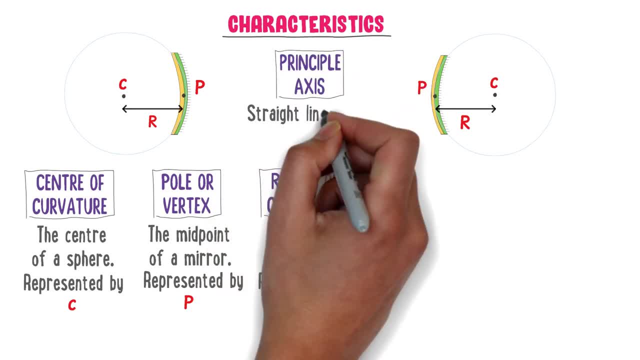 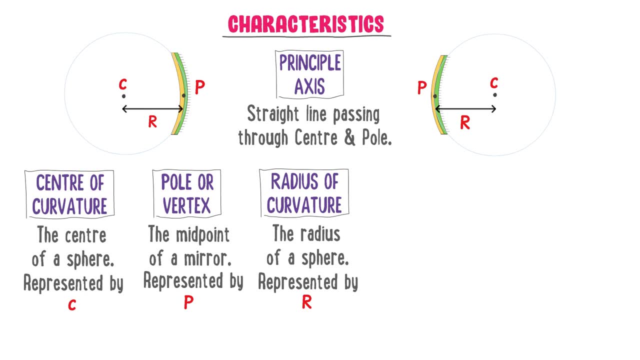 Fourthly, what is principal axis? The straight line that passes through the center and pole is called principal axis. For example, this line passing through the center of a curvature C and pole P is called principal axis of the concave mirror, While this line passing through the center of a curvature C and pole P is called principal axis of the convex mirror. 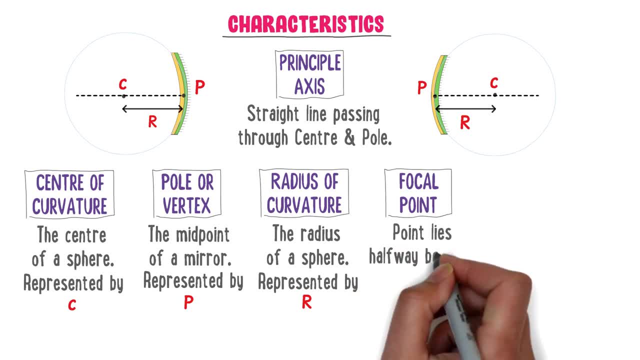 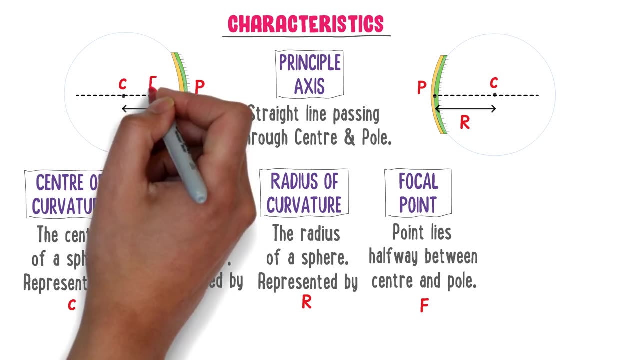 Fifthly, what is focal point? The point lies halfway between the center of curvature and pole is called focal point. It is represented by F. For example, This is the point between center of curvature and pole. so it is the focal point F of the concave mirror. 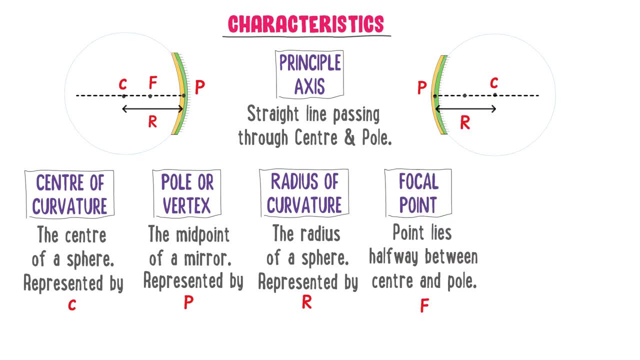 This is also the point between center of curvature and pole, so it is the focal point F of a convex mirror. Sixthly, what is focal length? The distance from the pole P to focal point F or the distance from the center to the focal point is called focal length. 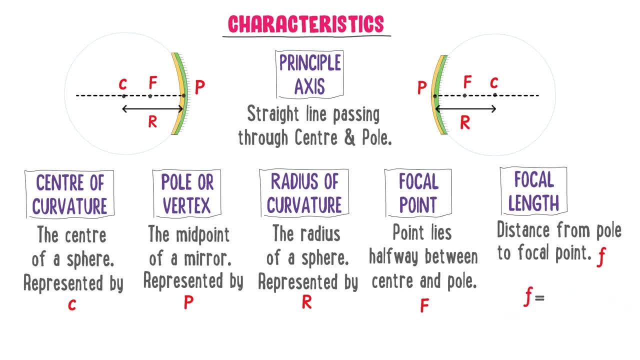 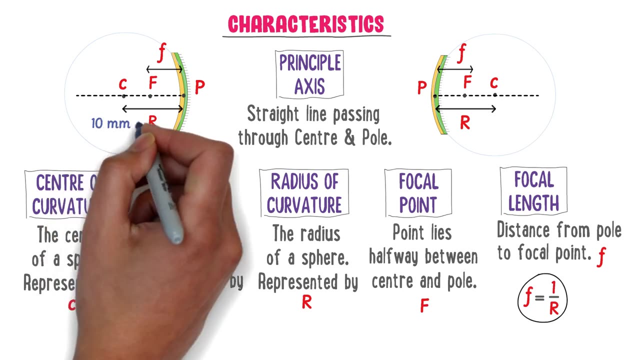 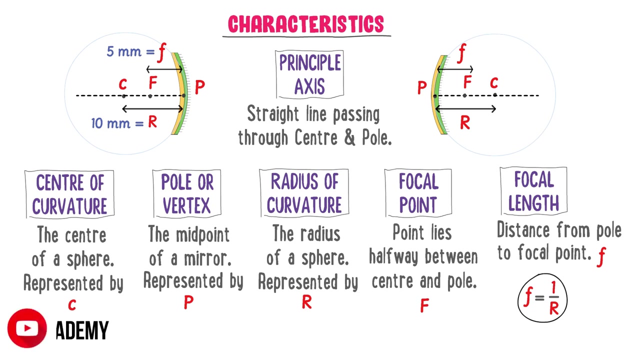 It is represented by small f. For example, For example F is equal to one half the radius, For example f, of a concave mirror, and this is the focal length F of a convex mirror. If the radius of a concave mirror is equal to 10 mm, then its focal length f is equal to 5 mm. 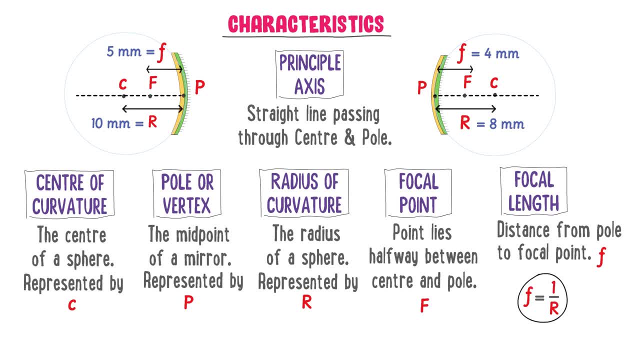 f of a convex mirror is equal to 8 mm, then its focal length is equal to 4 mm. So focal length F is equal to 7 mm. f is equal to half of radius. Here let me teach you two conceptual MCQs. 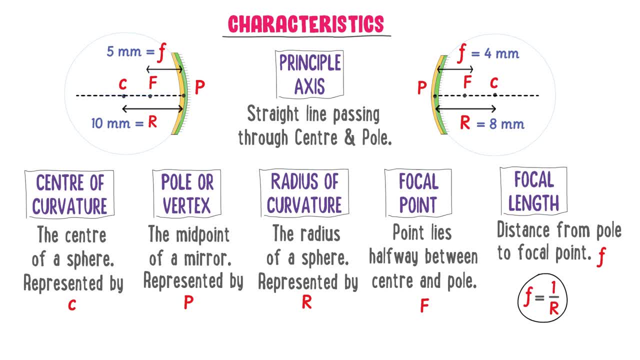 Firstly, center of a curvature and focal point lie at the same side of a reflecting surface of a concave mirror, while center of curvature and focal point lie at opposite side of the reflecting surface of a convex mirror. Secondly, principal axis intersects the mirror at 90 degree. hence noted down these MCQs. 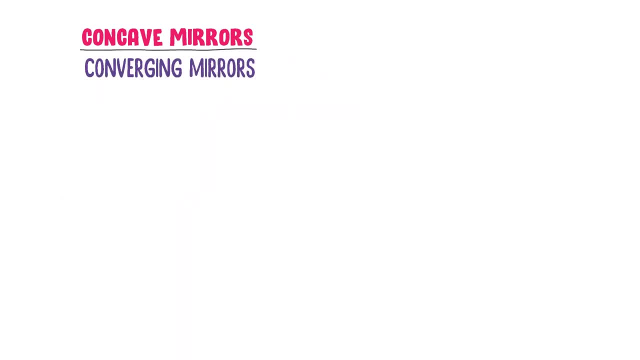 Finally, why concave mirrors are called as converging mirrors and why convex mirrors are called as diverging mirrors. Well, the word converge means come together or join together. Consider a concave mirror. When light beam falls on a concave mirror, after reflection, all the light rays joined together are converge at one point.